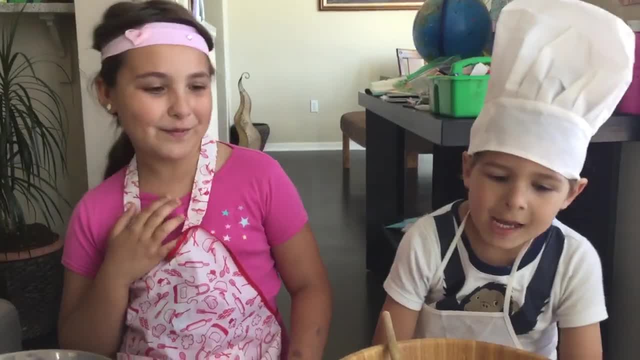 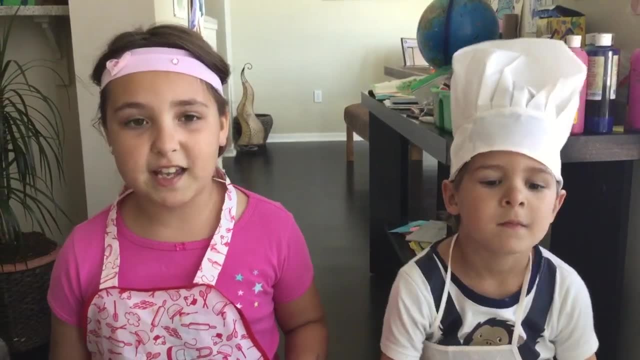 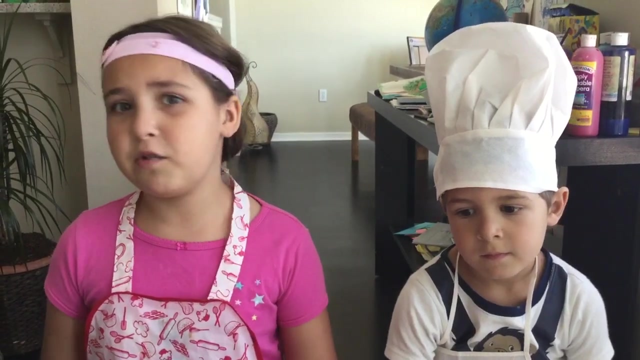 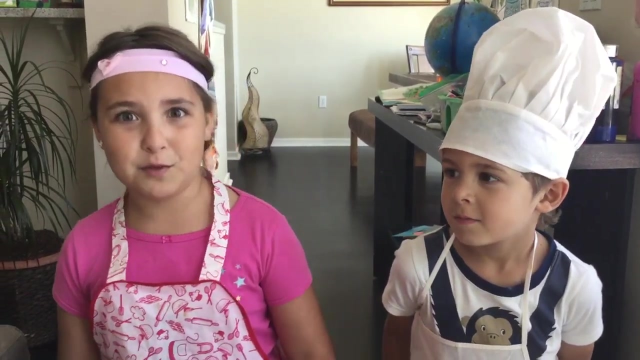 Hello everybody. My name is Layla and my name is Adam, and today we're going to be chefs. We're going to bake a yummy lemon cake. Now, my family and I are big chocolate fans, but this one, oh. it was delicious, And I have to warn you, you might lose self-control once you bake this. 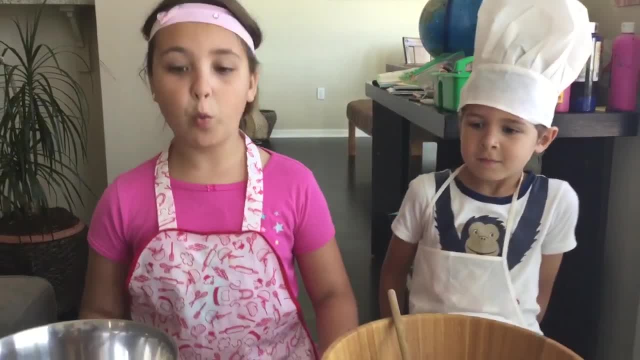 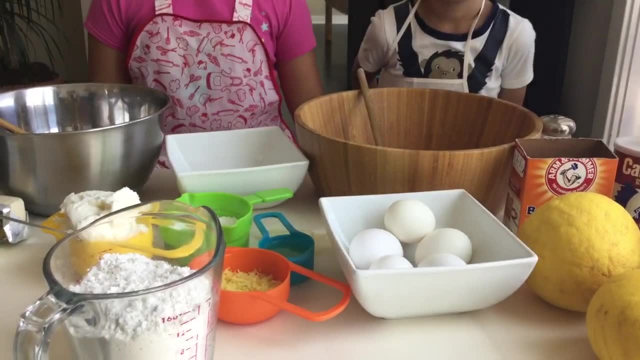 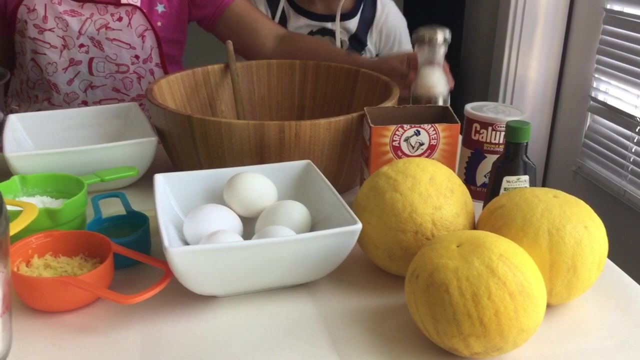 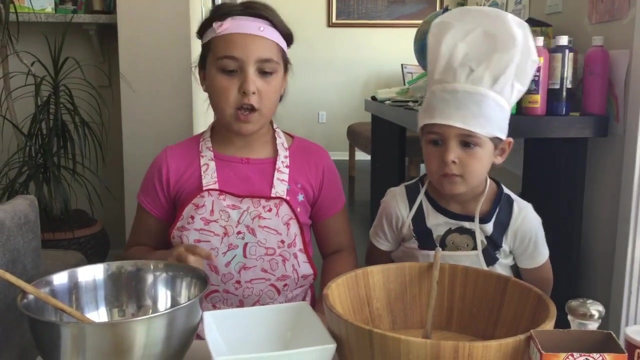 So let's get started. What you need is two cups of flour, one teaspoon of baking powder, half a teaspoon of baking soda and a pinch of salt, And that's going to be in bowl one. In bowl two, you need half a stick of butter. 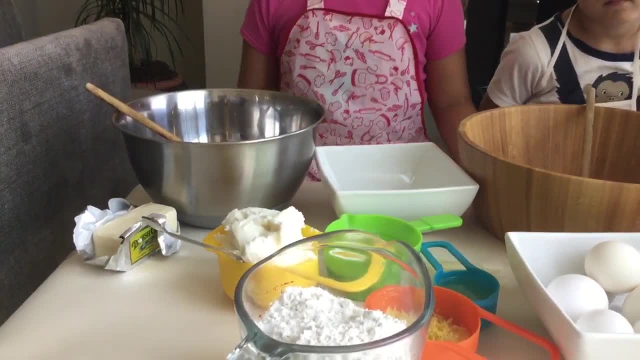 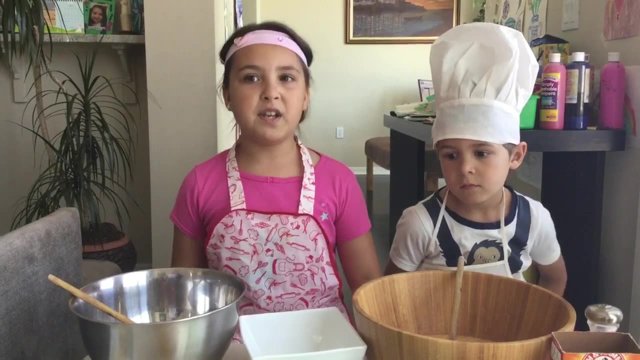 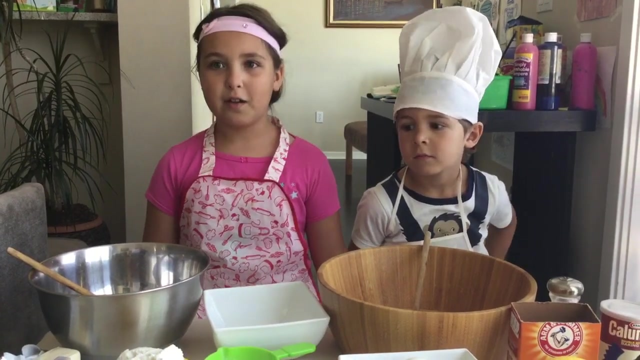 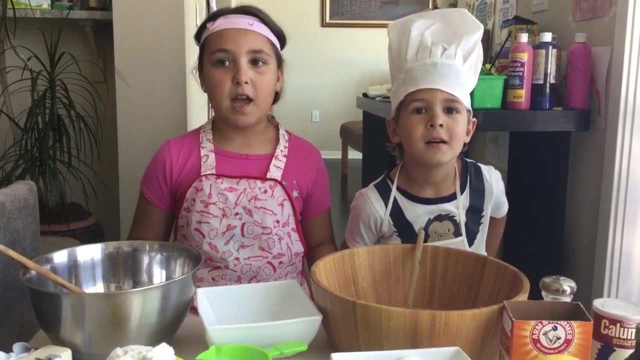 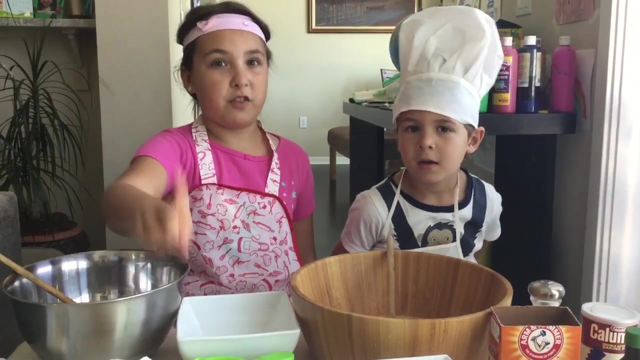 which is room temperature. Four teaspoons of lemon zest, one cup of sugar, one teaspoon of vanilla, five eggs, Five eggs- Can you believe that That's a lot of chickens? One fourth of cup of lemon juice, and then mix the two bowls and then add one and a half cup of. 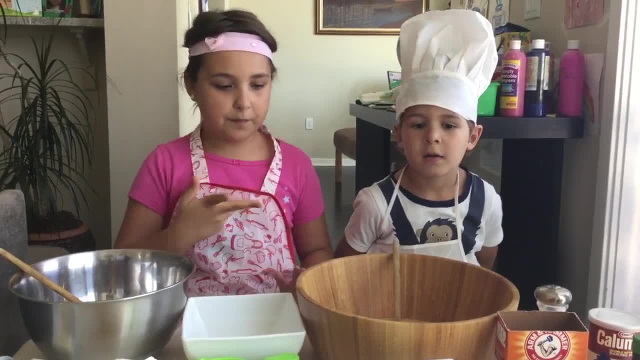 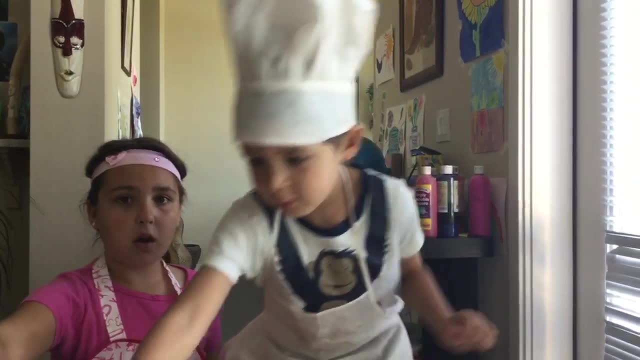 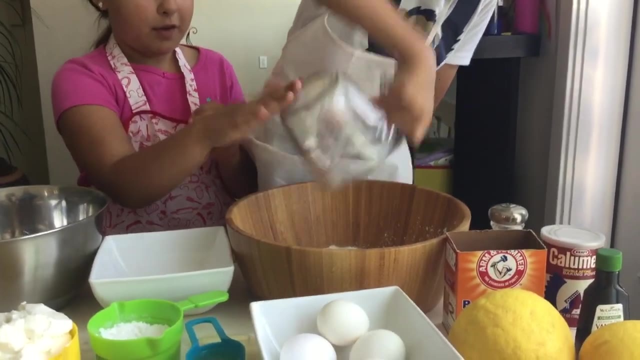 ricotta cheese. Now let's get started. In bowl one, add the flour. I'll add the flour, since it's bowl one. Aw man, it's your bowl, Darn it. Add a whole lot of flour. Come out there, flour. 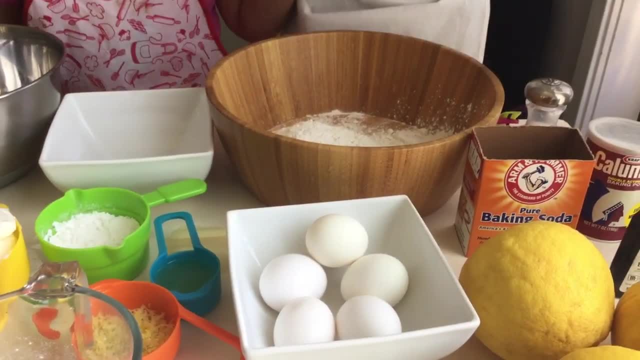 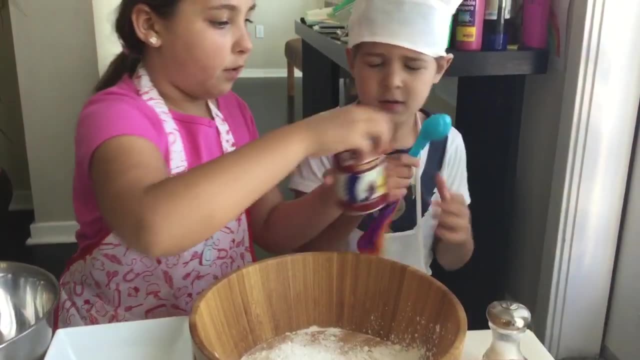 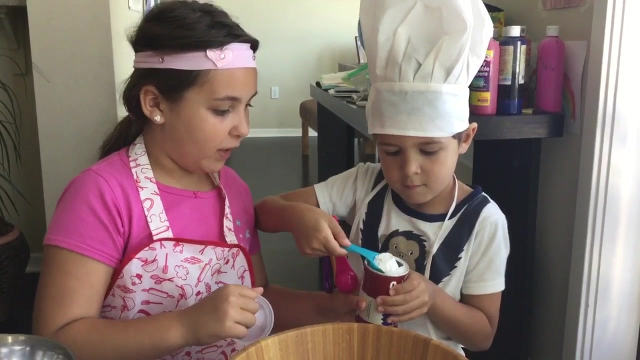 Next add the baking powder. Yikes, We're gonna use the blue spoon. We're going to use the blue spoon with the baking powder. Come on, Oh boy, Don't spill. Don't spill Super close. Yes. 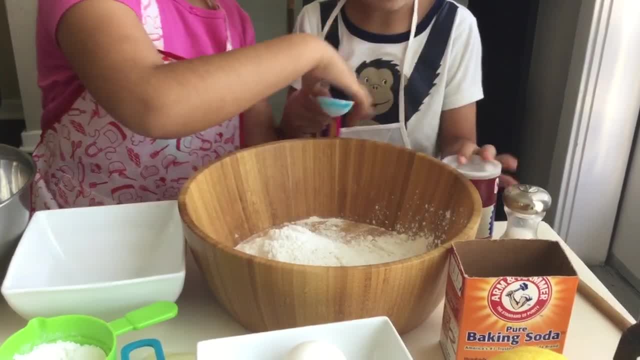 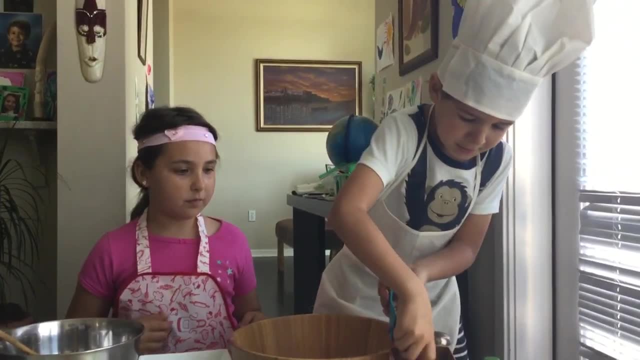 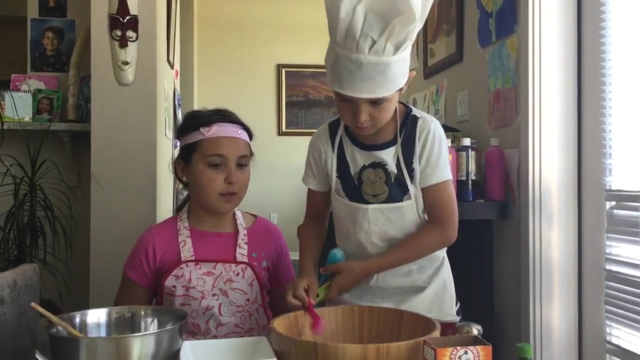 That was good. Next, let's add, with the pink spoon, some baking soda. Baking soda, Don't worry, You're about to do other stuff too Well, if you have one sibling, this cake is perfect because there are two bowls. 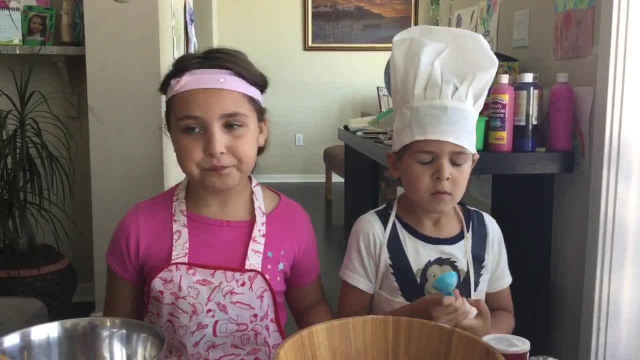 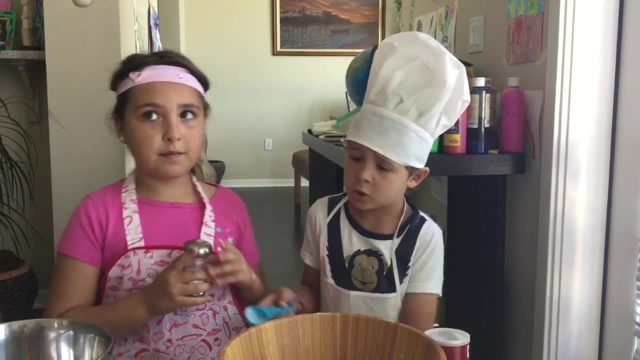 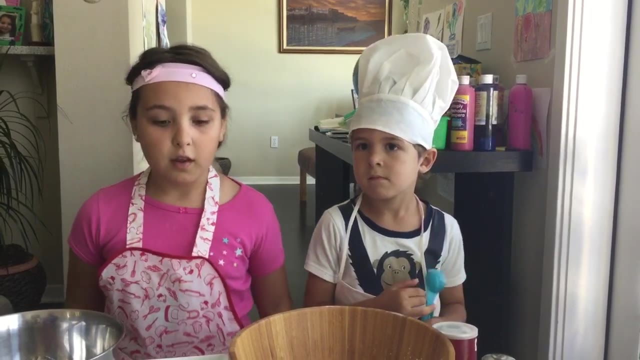 So you can do one bowl and your sibling does the other. Next, we're going to add the salt. Can I add the salt please? Sure, I think that's enough. Let's not add too much salt. Next in my bowl, we're going to add the butter. 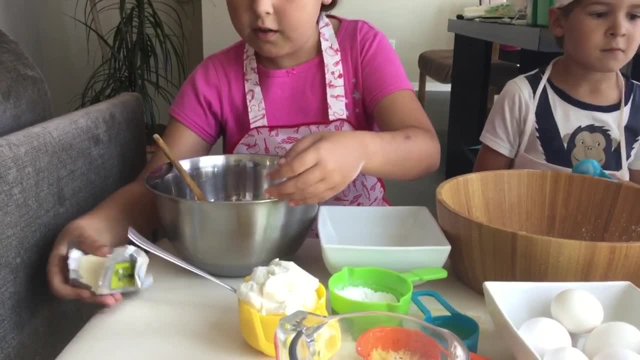 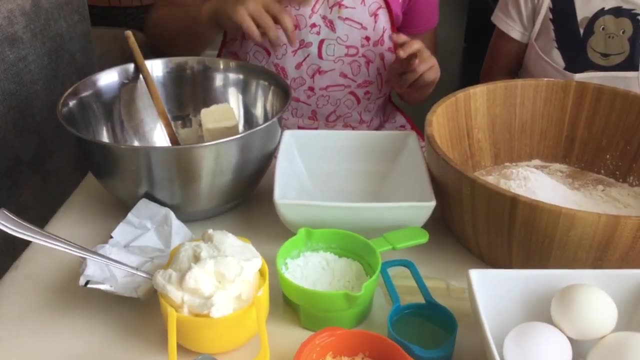 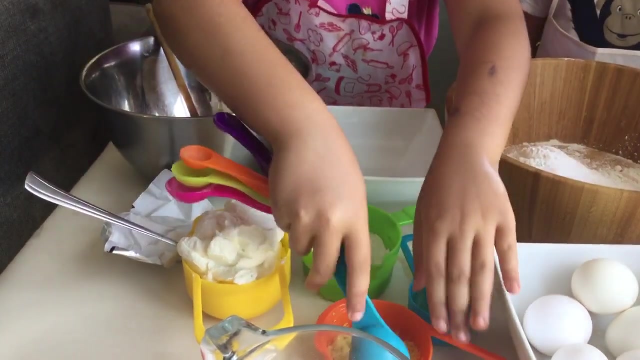 Oh boy. Where did the butter go There? it is There we go. Next, we're going to add four tablespoons of lemon zest. Adam, can I have it please? Thank you, Okay, One, Oh boy. 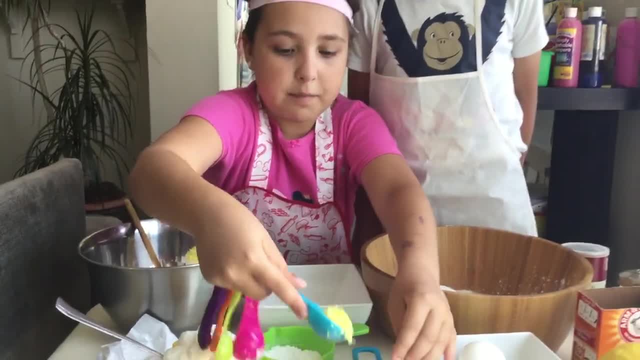 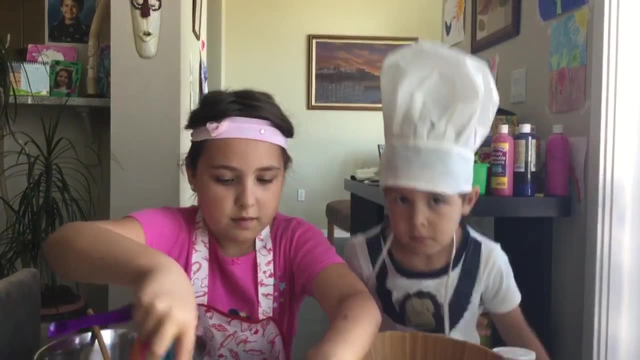 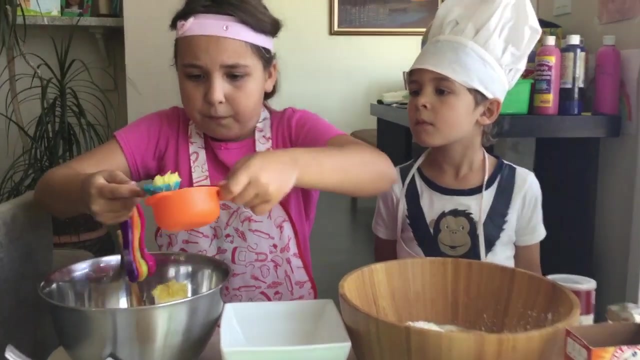 Shouldn't we just pour it in already? No, because it might not be exact. We have to be exact with our measures to make the cake absolutely divine. Okay, Three And four. Nice, I can smell the lemons already. 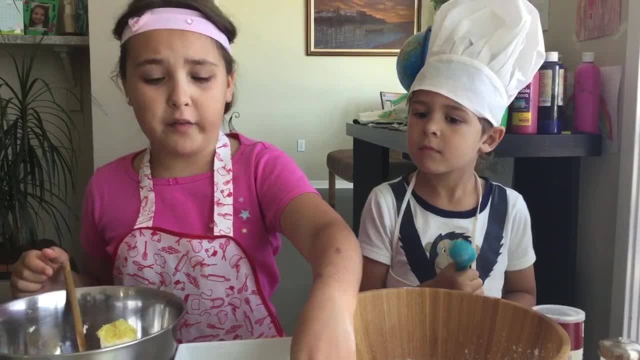 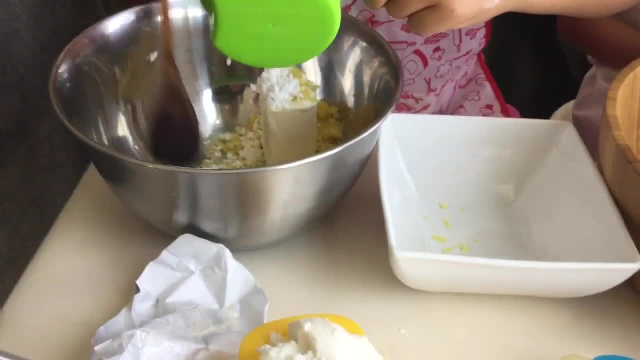 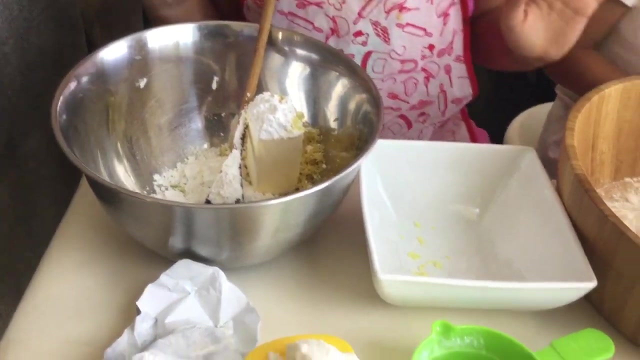 Thank you very much. Now let's add the cup, The cup of sugar, Mm, The best part. Come out the sugar. Oh no, It's stuck There we go. Next, we're going to add the one tablespoon of vanilla. 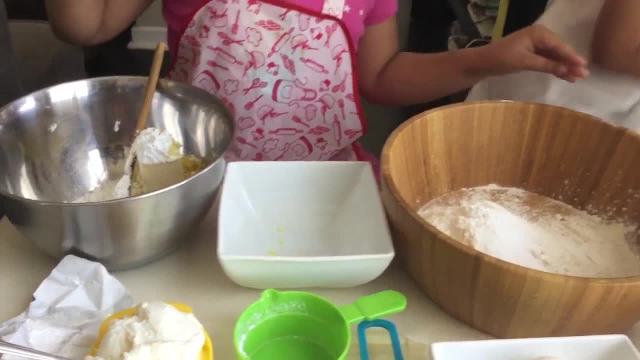 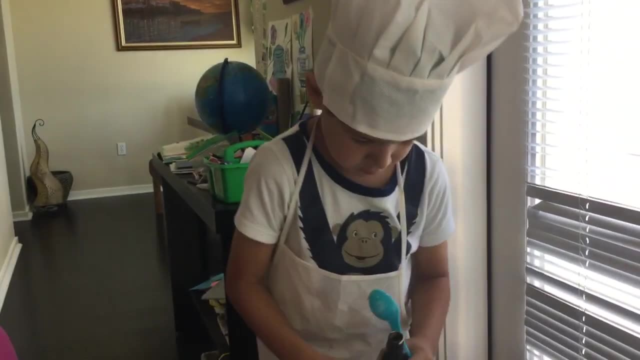 Now I'll do the vanilla Tick-tock, tick-tock, Let's go a little faster. They want to bake their dough. Oh my goodness, I'm going to add the vanilla. Oh my goodness, I'm going to add the vanilla. 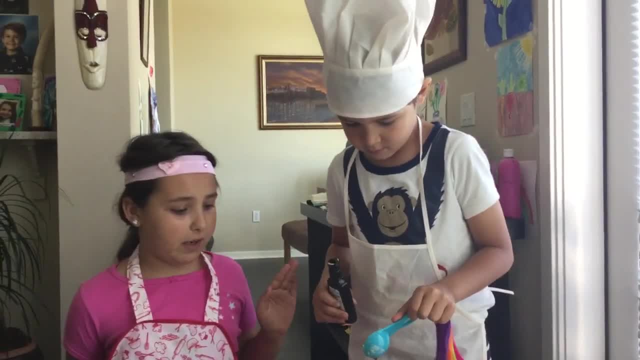 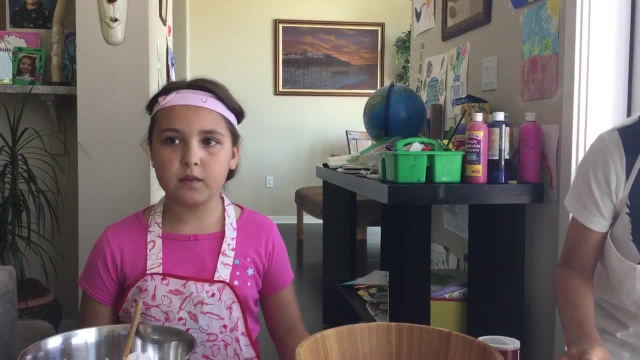 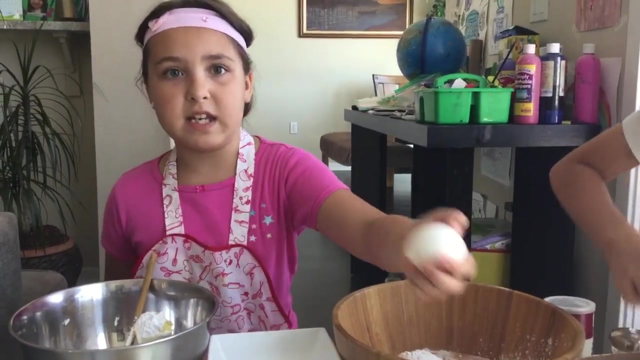 I'm going to add the vanilla. I'm going to add the vanilla. Oh, my goodness, Delicious cake already. Next, we're going to add the five eggs. We're going to add them in a separate bowl, so if we see a shell, we can take it out. 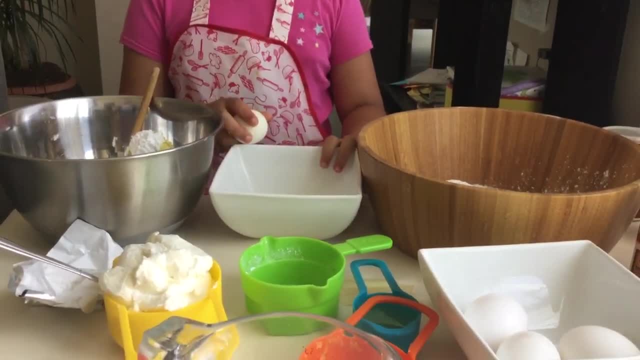 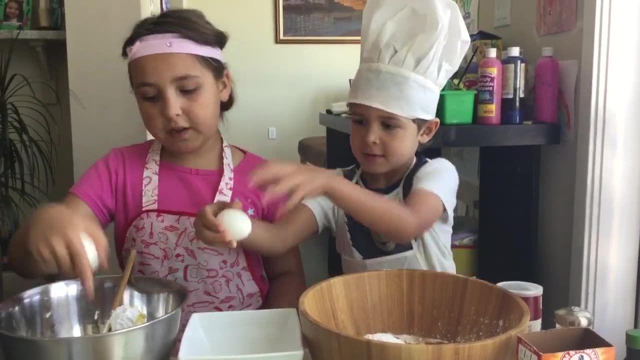 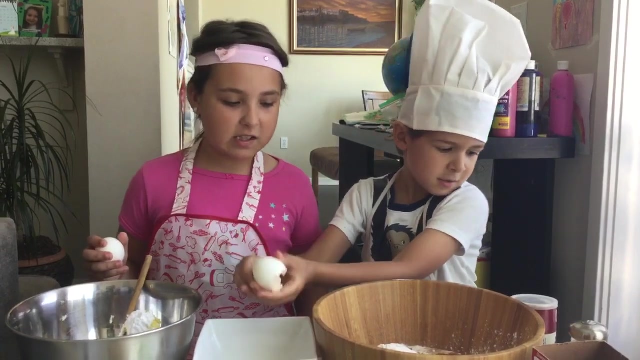 I'm going to do it. Remember, We made a deal, No, But I love doing the eggs. Sorry, And you did them yesterday. Don't forget to pour this in. pour it in this bowl. Oh, there's a shell, but we can take it out really easily, since we put it in. 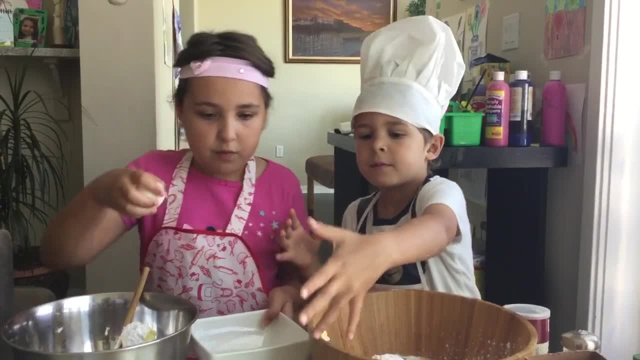 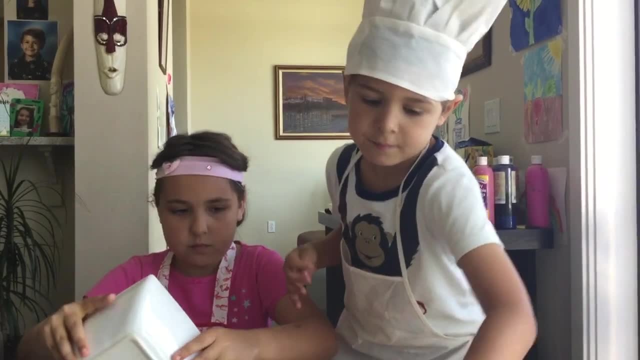 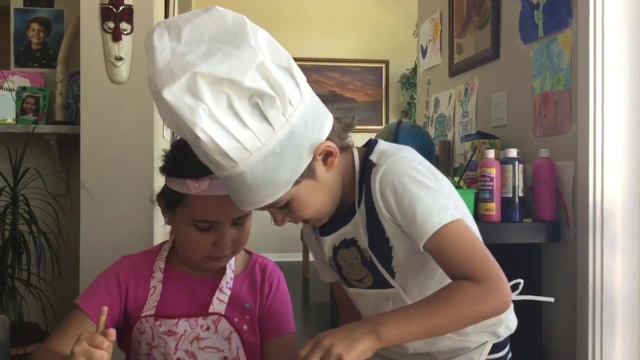 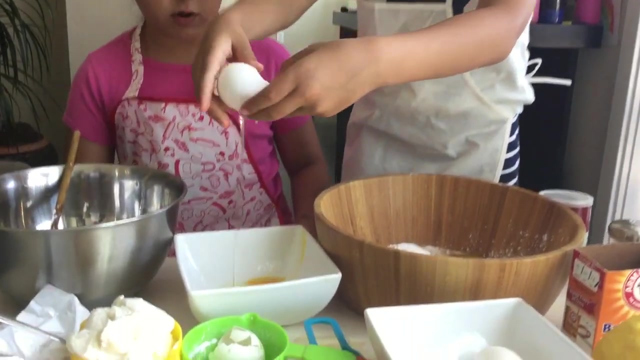 that bowl. Let's put them one at a time. Oh, Adam, don't make a mess. Put that egg in there. Now crack the egg, You can start mixing. Okay, Oh, that was close. Did you see that? Maybe I shouldn't trust him with the eggs anymore. 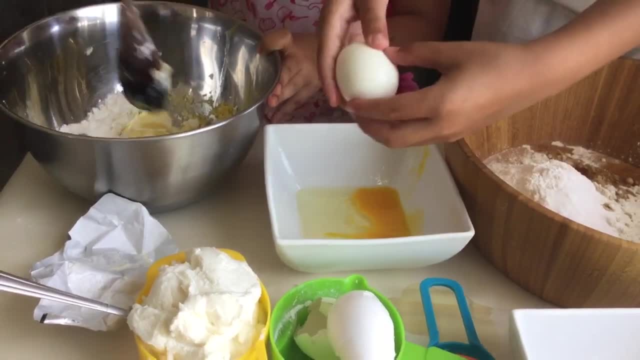 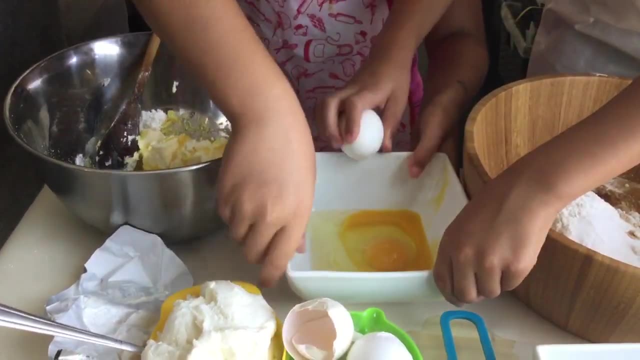 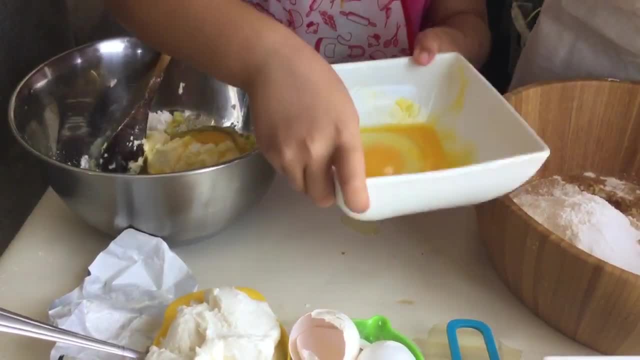 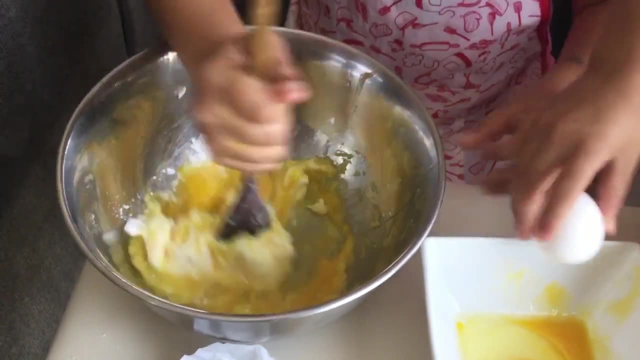 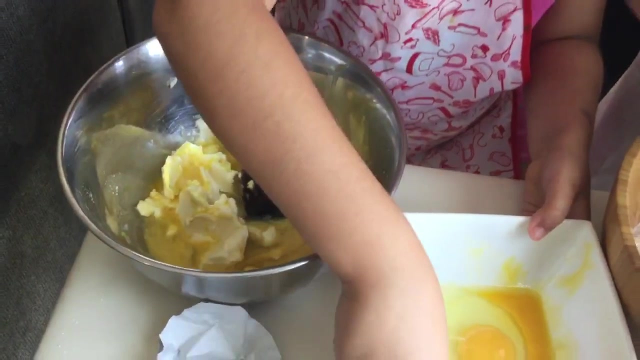 Well, let's do that. Don't crack another egg until I mix it up. Adam, please follow directions more. Adam, don't crack it up, please. I only want to get it started, then I'll crack it once you're done stirring, Now let's add this egg. Now you can put it in. 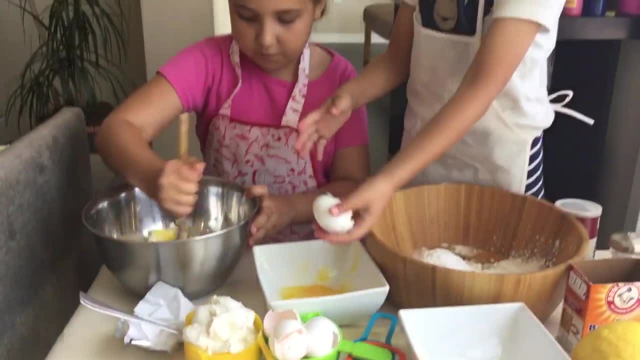 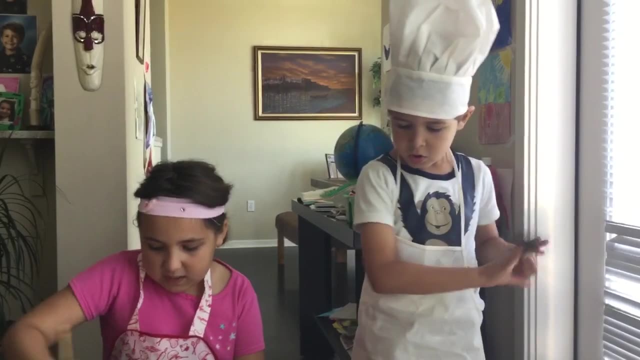 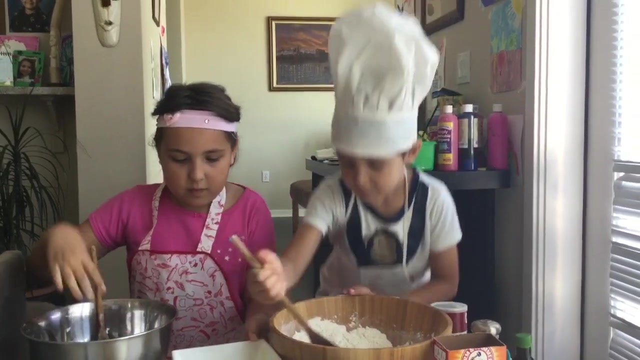 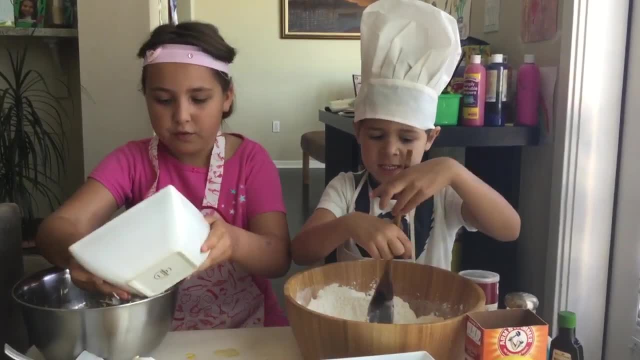 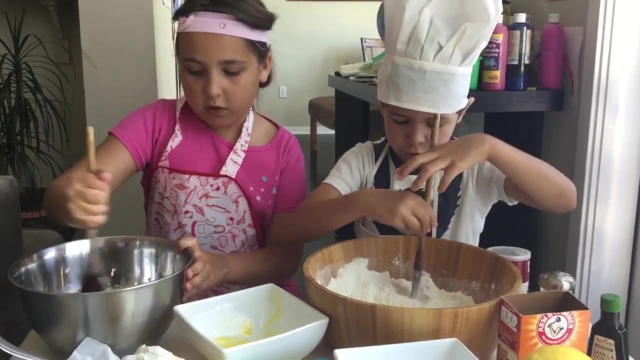 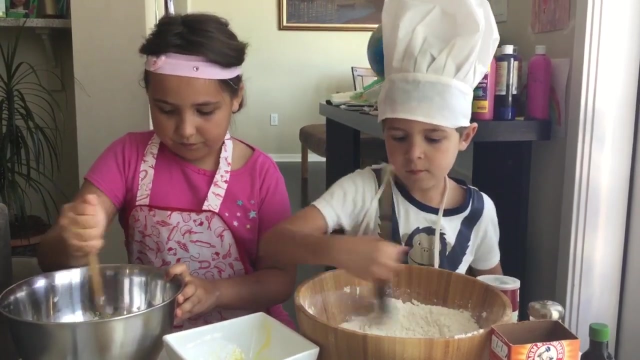 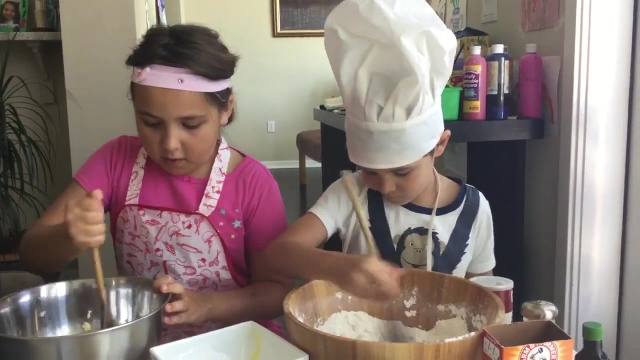 Finally, I'm going to add the last egg. Wow, I'm an electric mixer. Now mix until all the ingredients are mixed together, but make sure your sieve does not make a mess. This is a little messy. Good thing we have our aprons. Hmm, can you smell it? I can, and it smells. 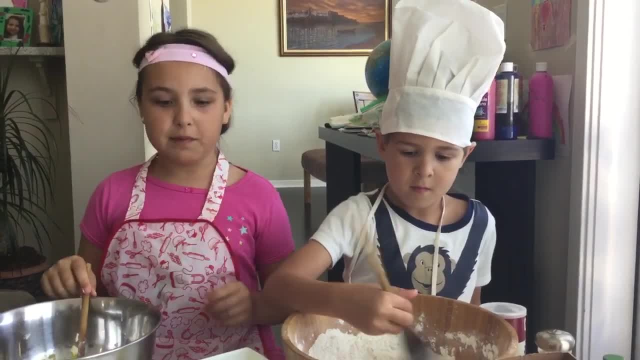 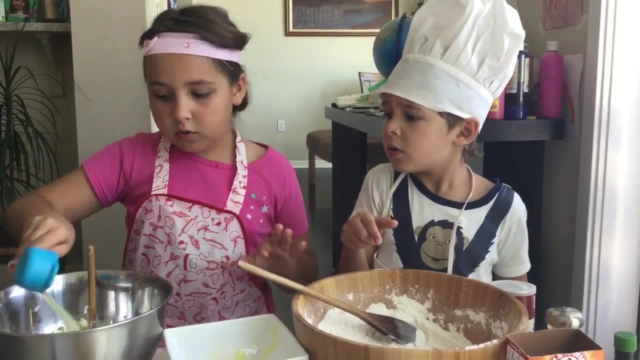 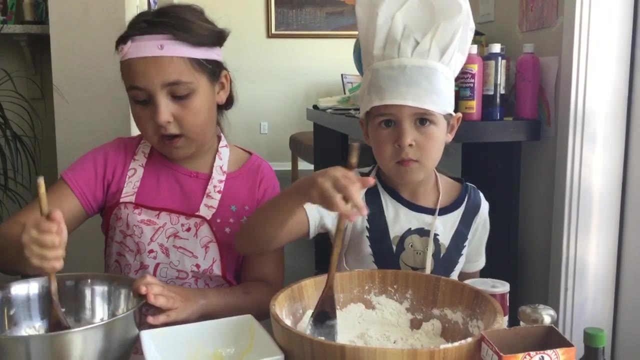 delicious. Now let's add a quarter cup of lemon juice. Ah, it's stuck to mine. We have to put it in this bowl, bowl two, or otherwise the cake won't work or turn out as good, And we don't want that right. 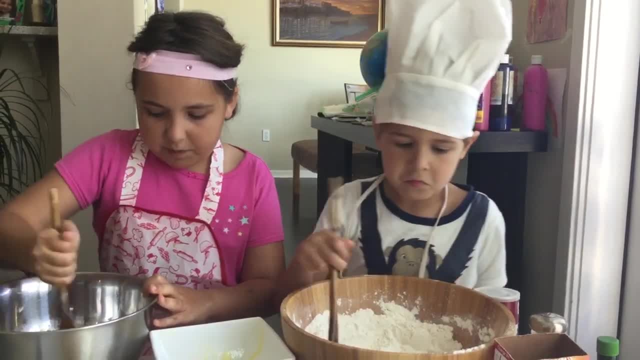 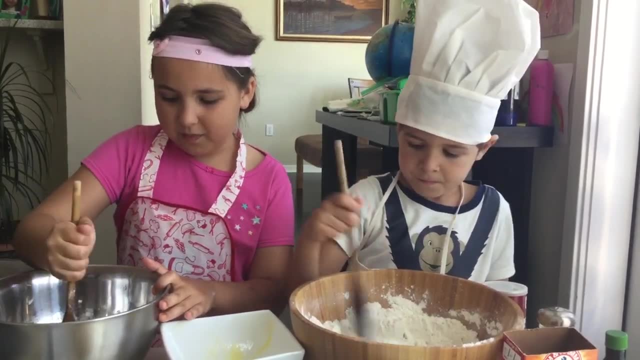 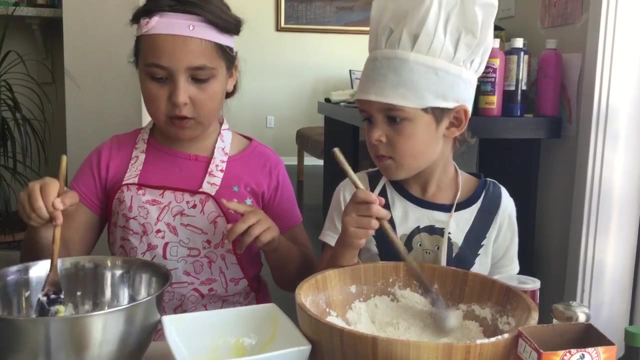 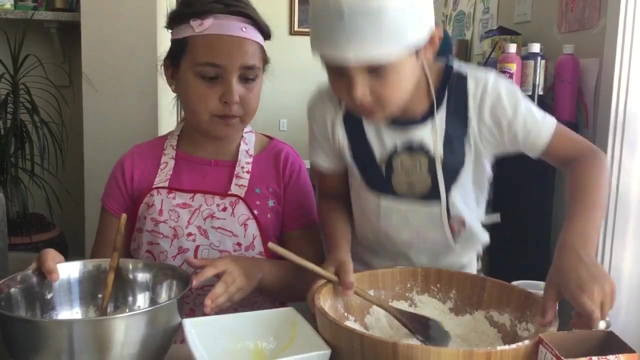 Okay, keep stirring, stirring, stirring. Ah, it's splattered on me. Now let's mix the two bowls. Hmm, which bowl are we going to pour it in? Pour your bowl into mine, and then we're going to mix, mix, mix. But it might get a little messy. Let's pour it in. 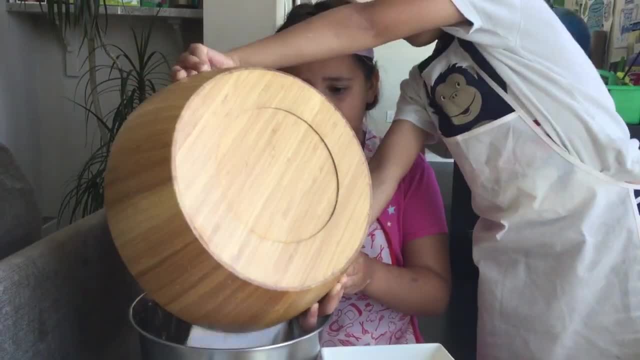 Oh no, Oh no, I kind of Don't spill. There's still a lot Yikes, Yikes. Let's put it with the spoon. But, Adam, you're shining in my spotlight. I'm sorry, but I. 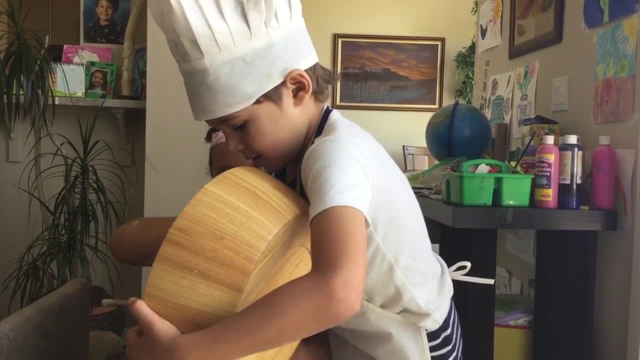 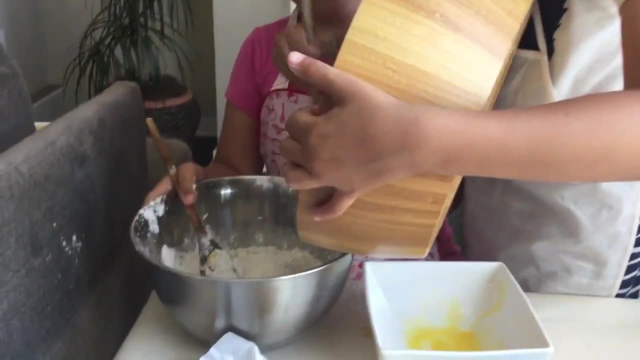 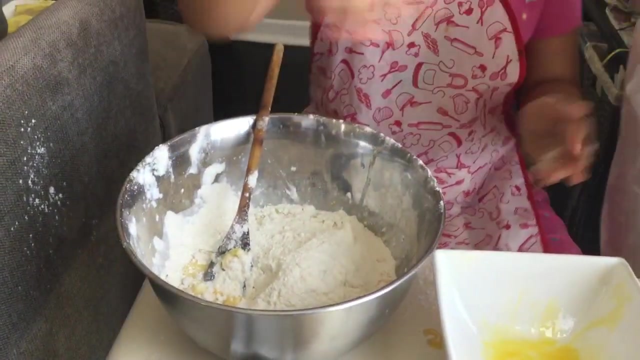 Adam, it's super messy. I think this is enough, Adam. No, Don't get it on the couch or Papa will kill us. He'll be so mad at us if we get it all over the couch. Yeah, maybe not. 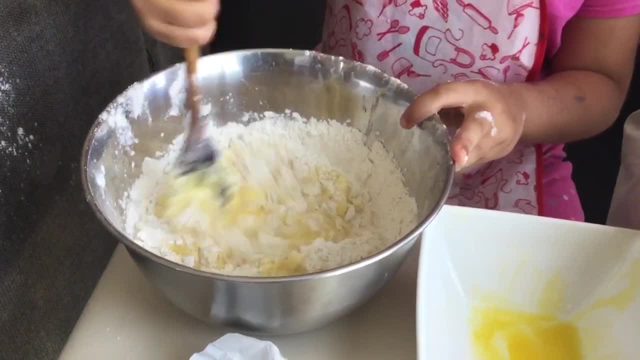 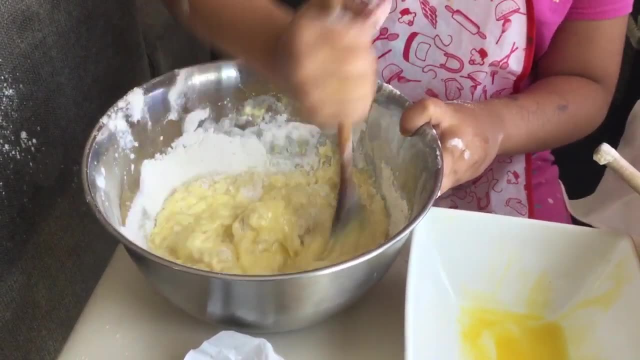 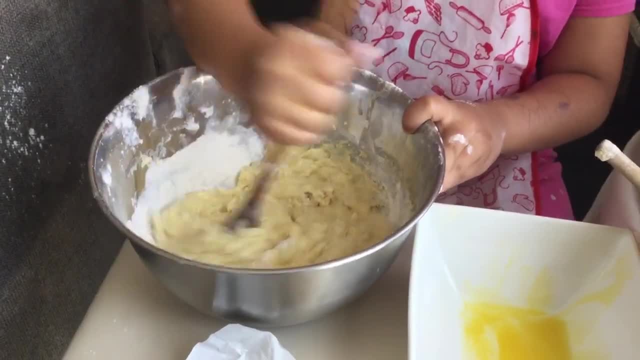 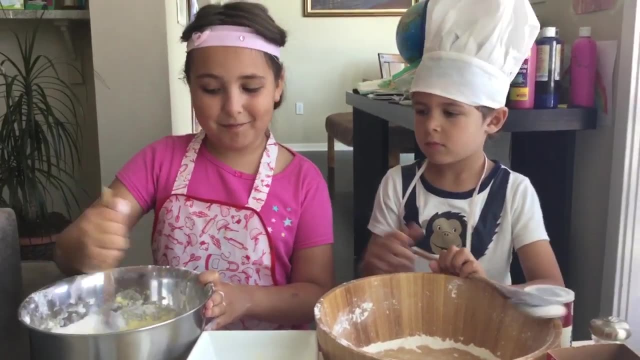 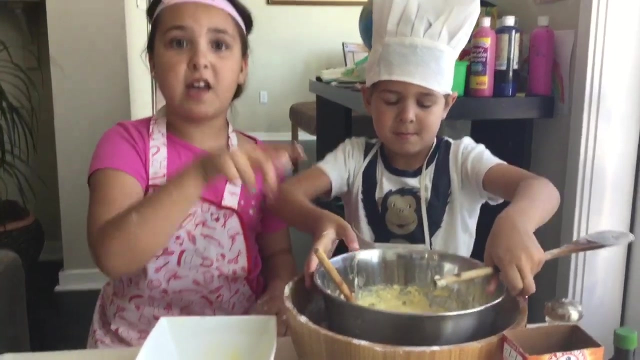 What? Oh man, But you were the one who made the mess. Fine, I'll let you mix next year, Oh man, Fine. Oh yeah, We can put it in the other, in the bigger bowl. So it's not going. 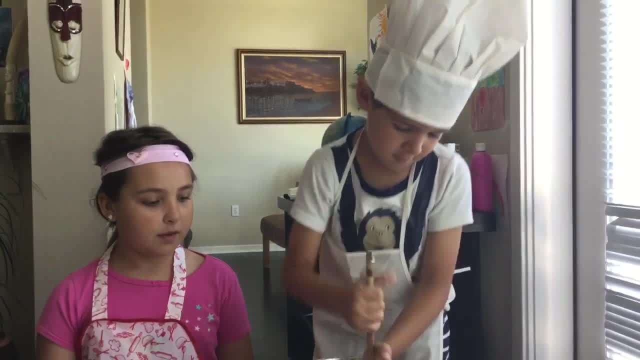 to splatter out as much. Let's both do it, so it's faster: Splat, splat, splat, splat, splat, splat, splat. Now the final ingredient: Let's add the ricotta cheese. 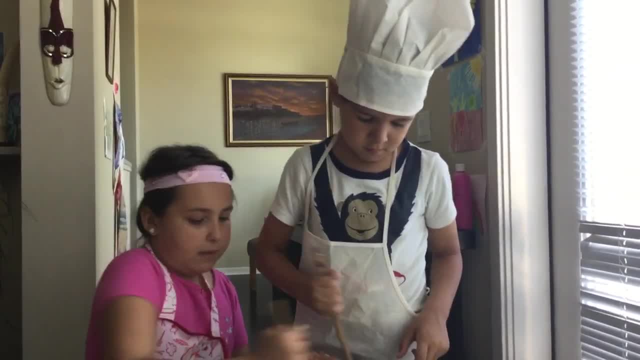 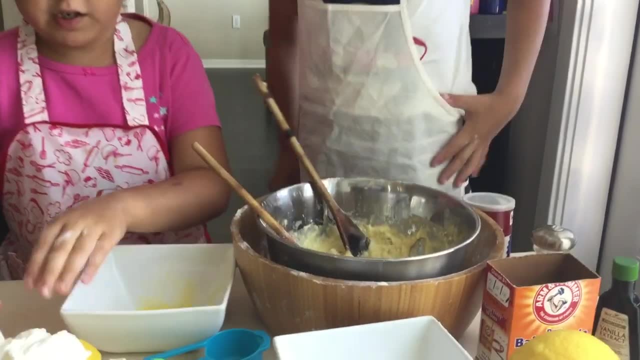 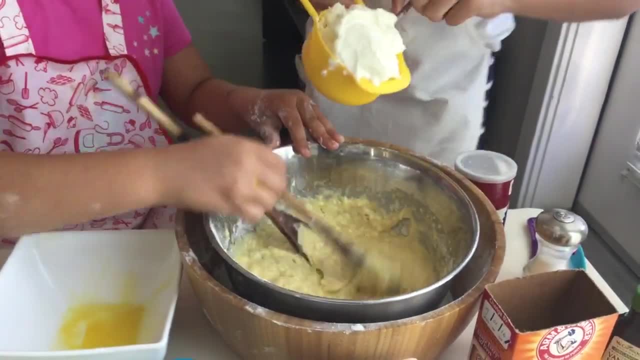 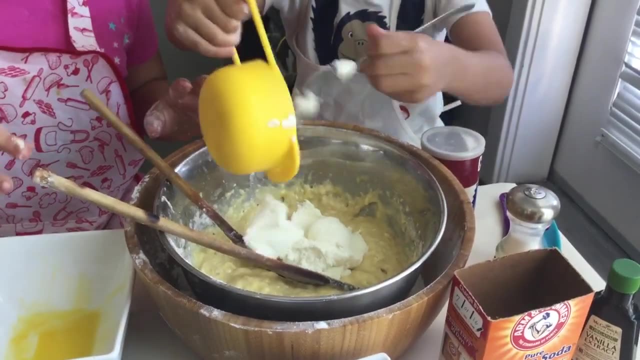 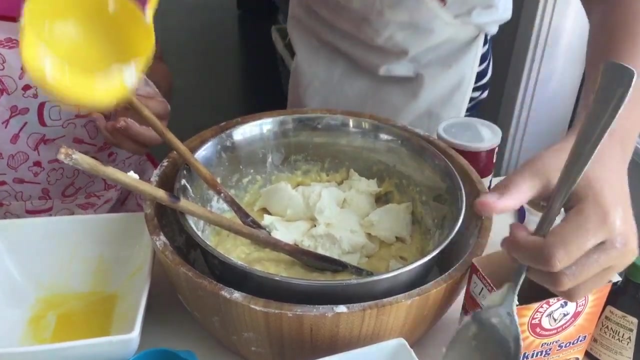 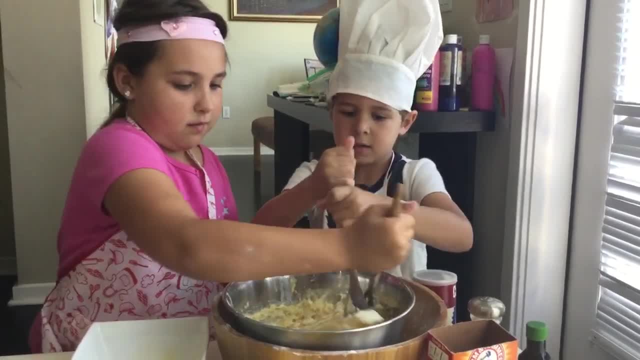 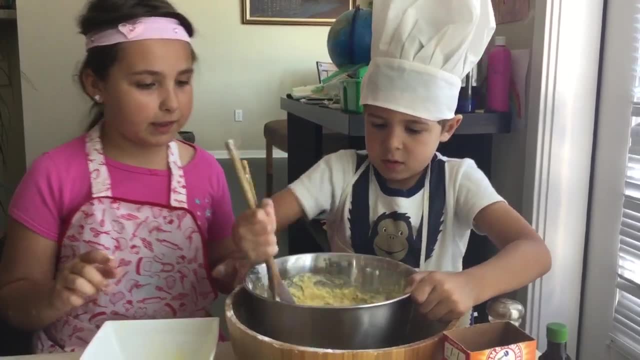 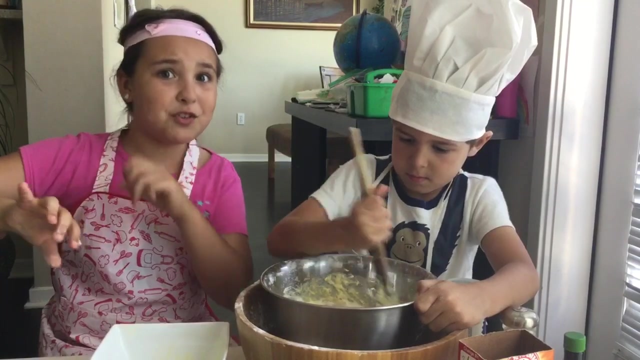 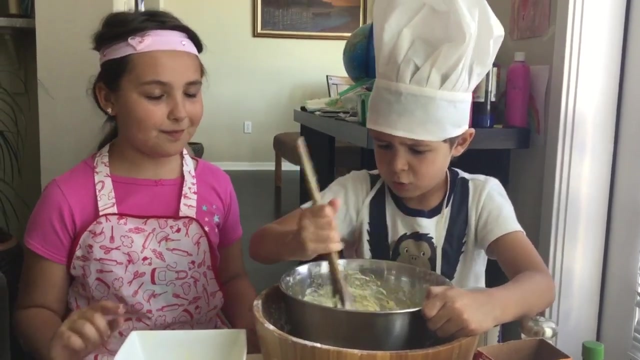 it's kind of whitish yellow. yeah, oh, man, stirring together is a little harder, but if you're simply left, then add the two spoons together and stir. it's kind of like a double mixer. wait, am i a little dirty here? oh, no, adam, you got me all dirty, i didn't. what are you talking about? 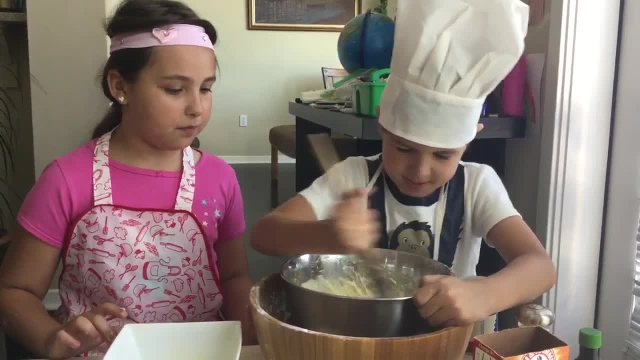 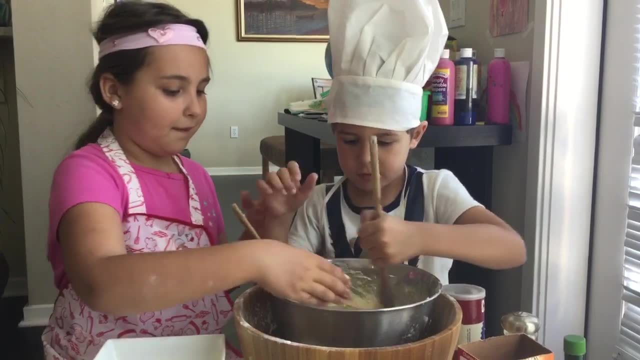 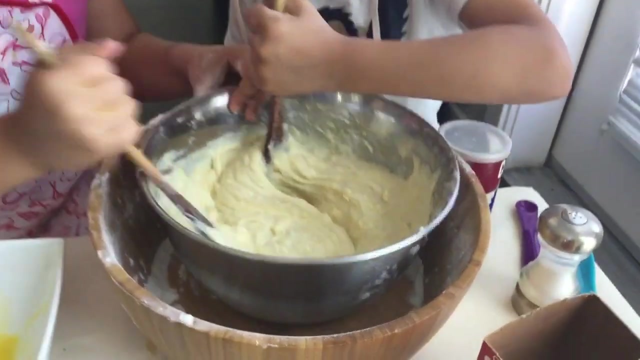 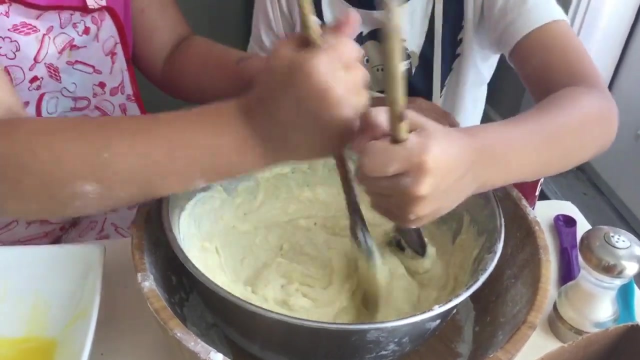 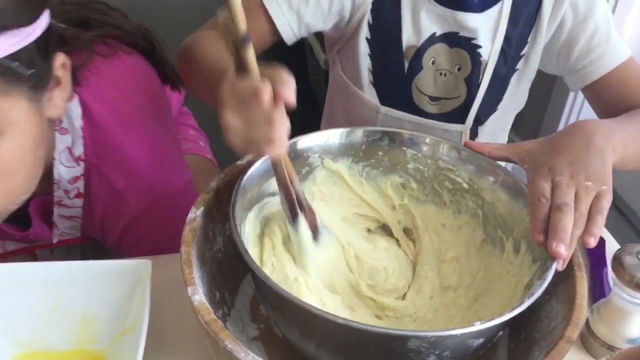 siblings gonna be fun, but sometimes hard. this is harder than i expected. please can i stir? it gets really sticky so you might want to ask an adult for help, like we did yesterday, but this time we're big kids and we're gonna do it by ourselves. now, when that's all ready- which i think it is right now- let's put it in this pan. 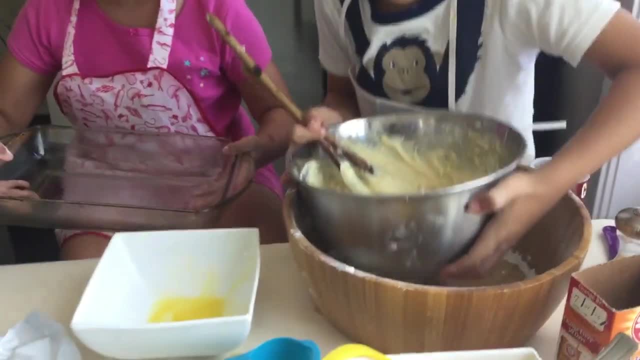 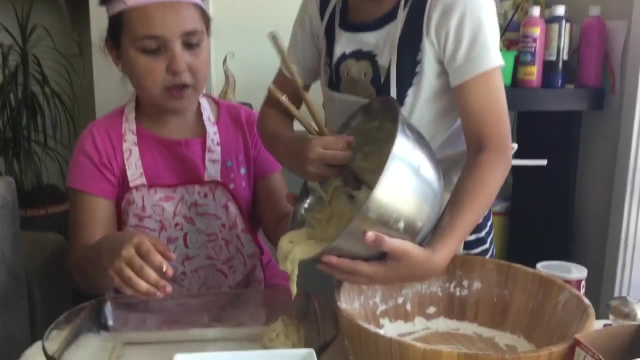 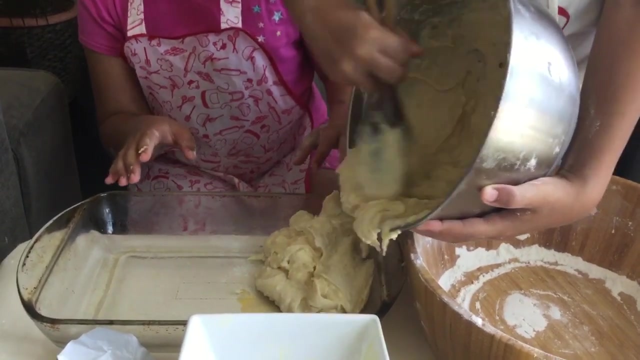 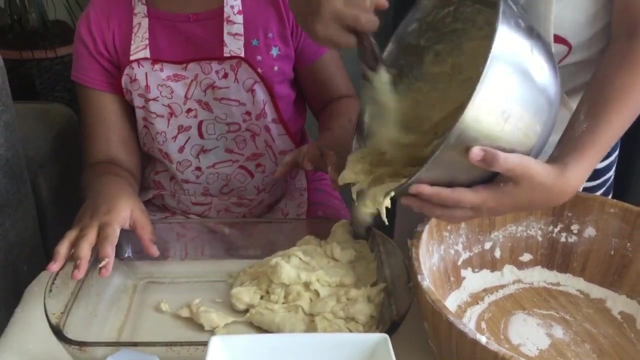 make sure you put some coconut oil on it. oh boy, maybe can i put it this time and then, when you're finished doing that, pop it in the oven for about 50 minutes, but first let's see if we can escape without making a mess. oh boy, this is just getting longer and longer. 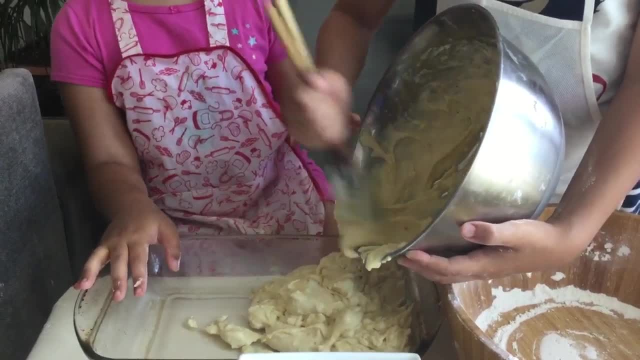 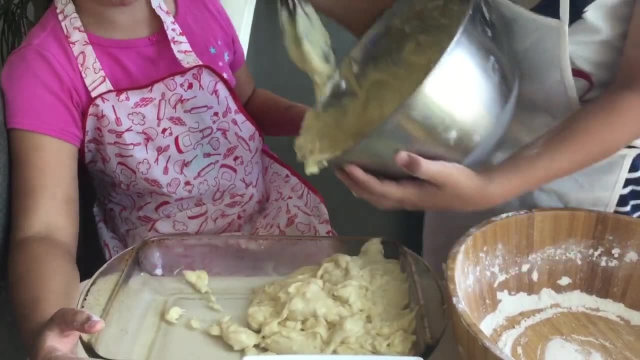 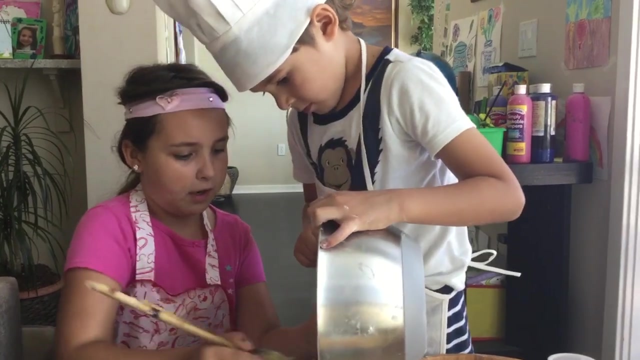 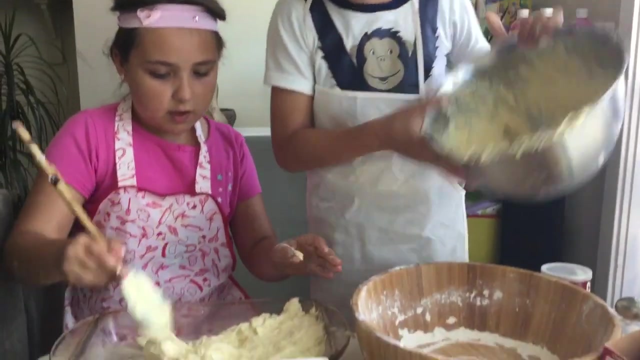 and i'm getting a little more nervous every passing second. please can i do it? well, i'm just done with this getting all messy. Good thing I have an apron on This could get messy, so best to put on an apron. You got most of the mixture out Now I'm going to do the rest, right? Yeah, fine. 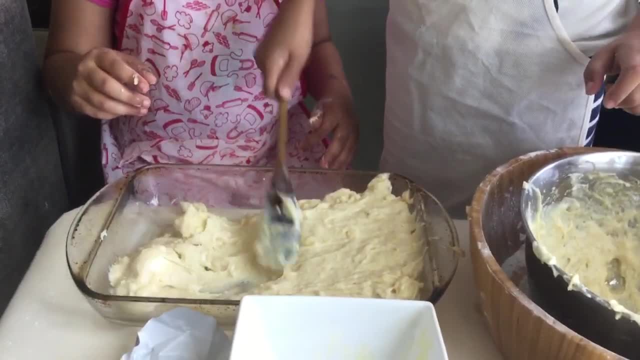 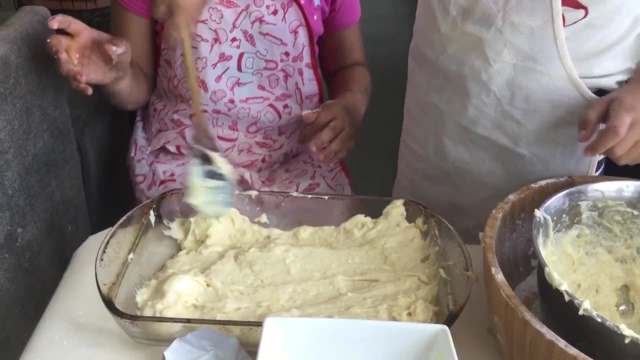 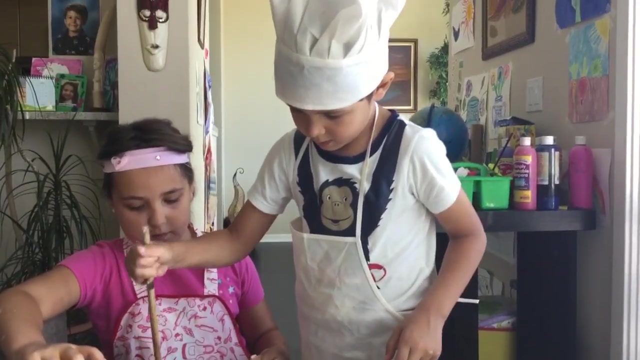 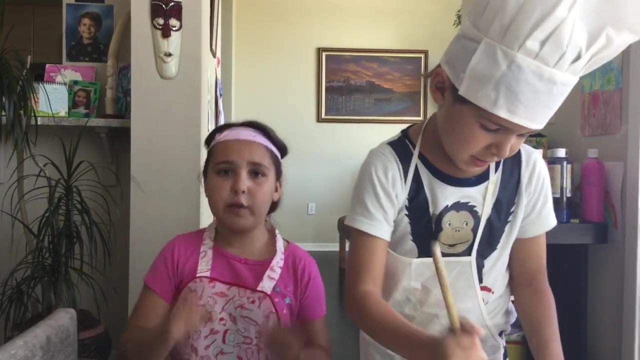 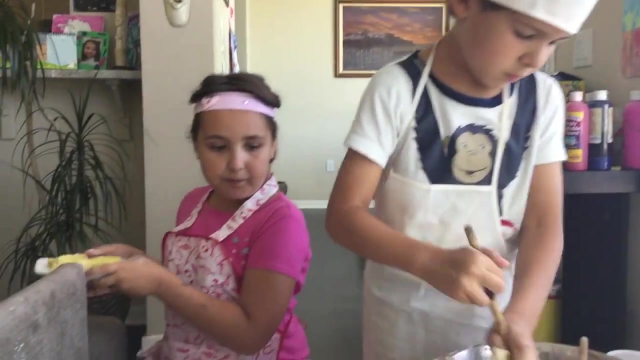 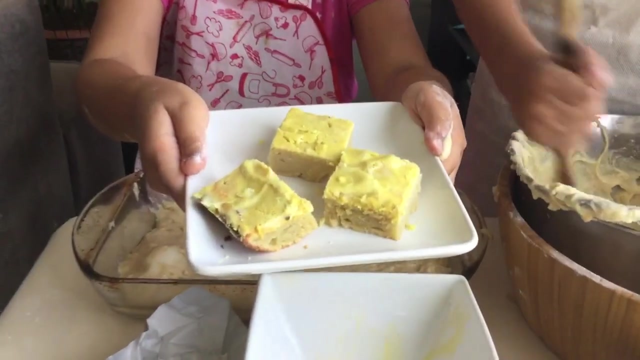 Spread it all out. Spread this all over the place, right, Yeah, And you can make some frosting with it, But after it's baked, I don't think we did some of it all correct. This needs to go back. Well, we don't want to keep you guys waiting, So after you pop it in the oven and put the icing on, that part's optional, before Adam bores you to death, this is our cakes. This is the result.